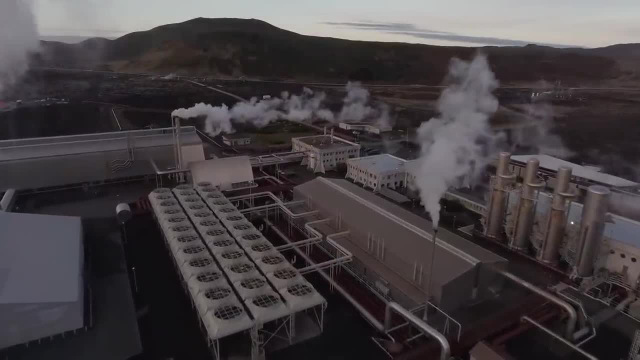 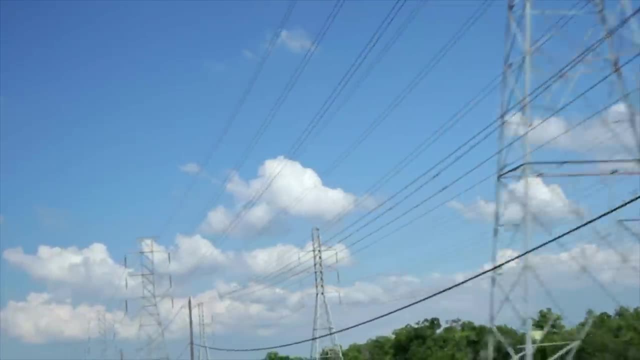 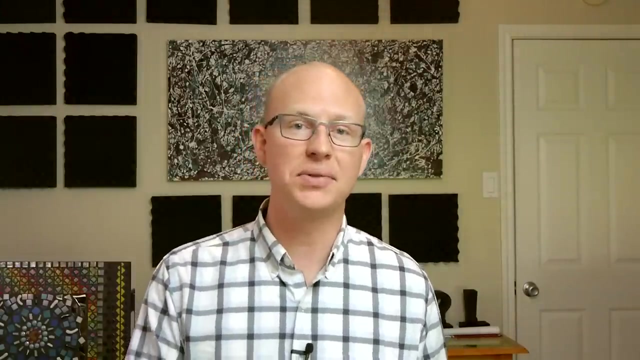 and most people don't like to live near large industrial facilities. That means massive amounts of electricity need to be transported long distances from where it's created to where it's used. Power lines are the obvious solution to this problem, and, sure enough, stringing wires, called conductors by power professionals, over vast expanses of rural. 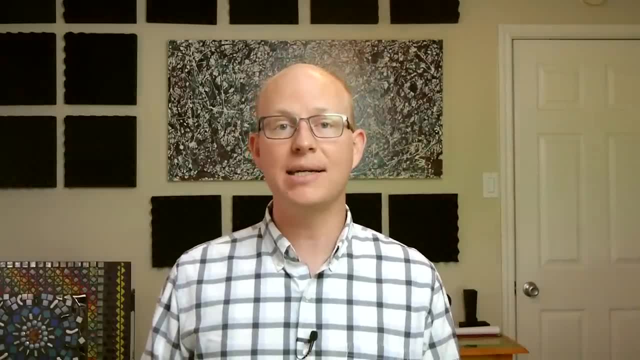 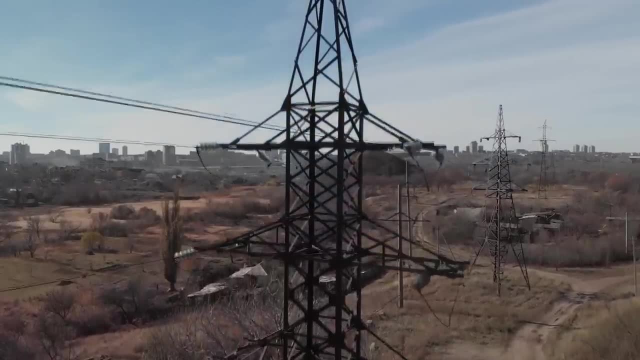 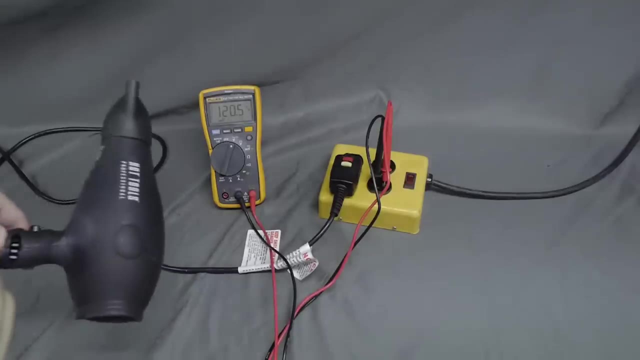 countryside is in general how the bulk transport of electricity is carried out. But if we want that transport to be efficient, there's more to consider. Even good conductors like aluminum and copper have some resistance to the flow of electric current. You can even see this at home. We can measure a small drop in voltage when 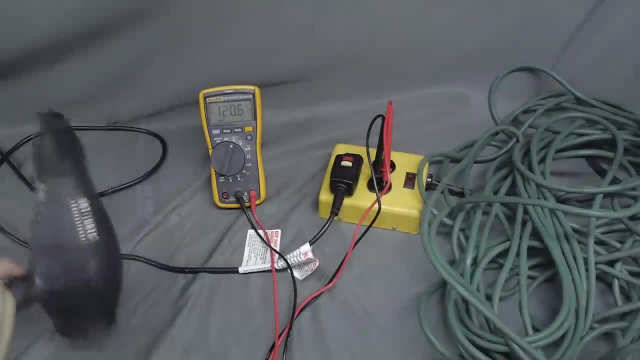 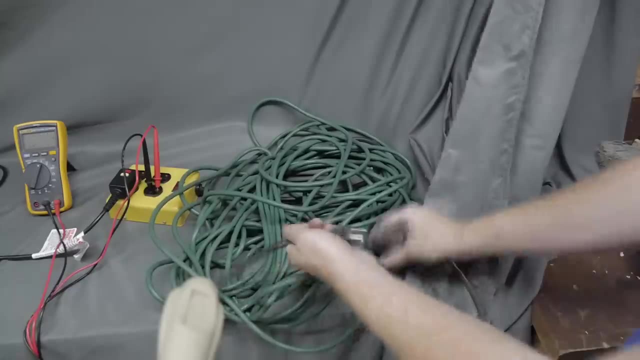 a hairdryer is plugged in directly to an outlet and turned on, Trying this again at the end of a long extension cord, the drop in voltage is much more significant. This difference in power represents energy lost as heat from the resistance of the extension. 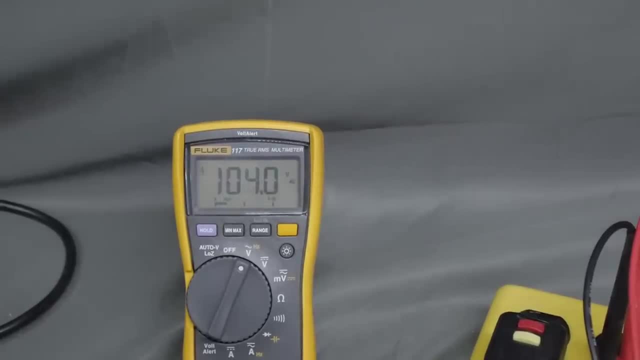 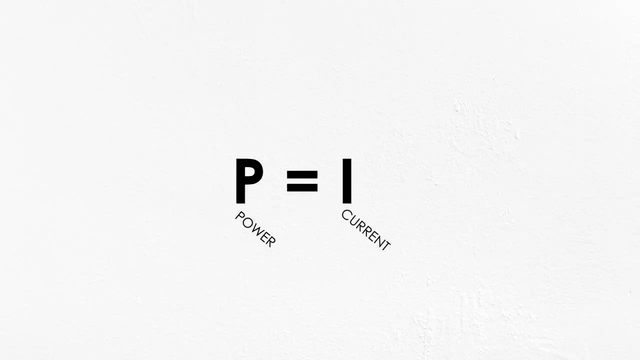 cord. In fact, this lost power is pretty easy to calculate if you're willing to do a little bit of algebra, which I always am. Electrical power is the product of the current, that's the flow rate of electric charge, and the voltage, that's the difference in electric potential. 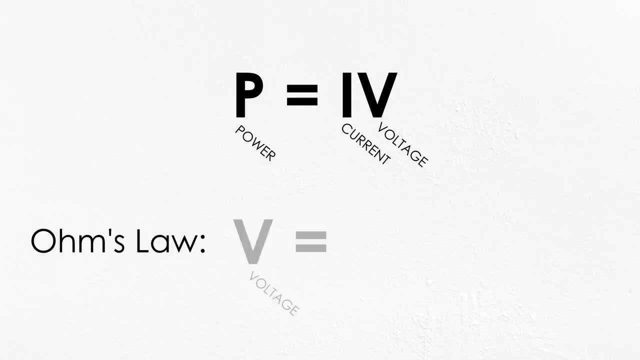 For a simple conductor. we can use Ohm's law to show that the drop in voltage from one end of a wire to the other is equal to the current times the resistance of the wire measured in ohms. Substituting this relationship in, we find that the power loss is equal to. 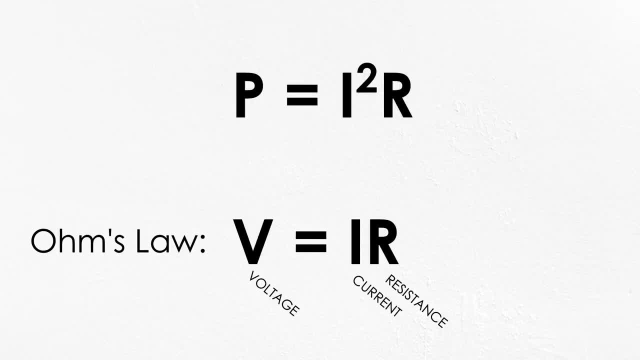 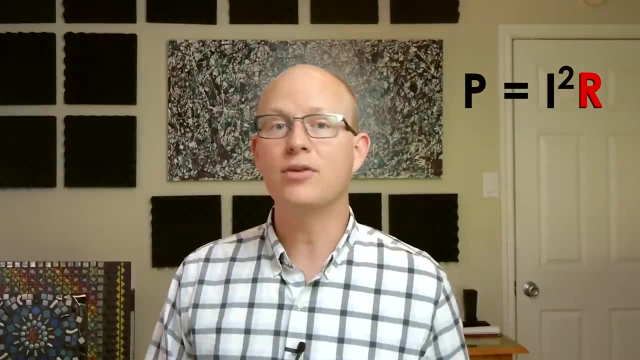 the product of current squared and resistance. So if we want to reduce the losses in a power line, we have two variables to play with. We can reduce the resistance of the conductor by increasing its size or using a more conductive material. but look at what matters more: the 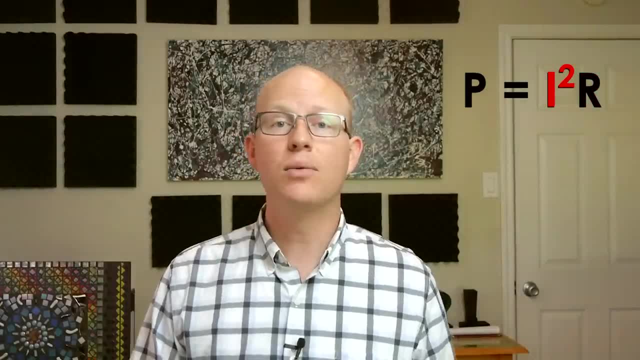 I squared term. Reducing the current by half will cut the lost power by half. That's the difference between the current and the resistance of the wire. We can also reduce the resistance of the wire by increasing the resistance of the wire by one, fourth and so on. Going back to Ohm's law, we can see that the only way 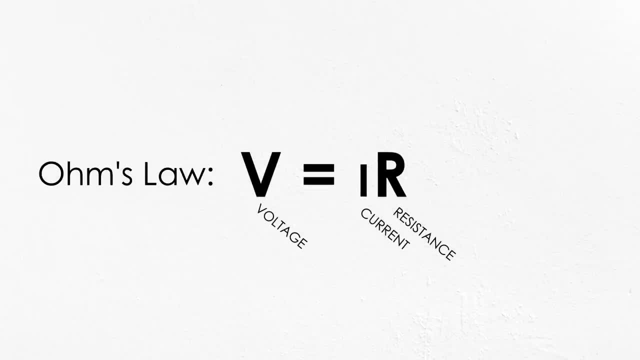 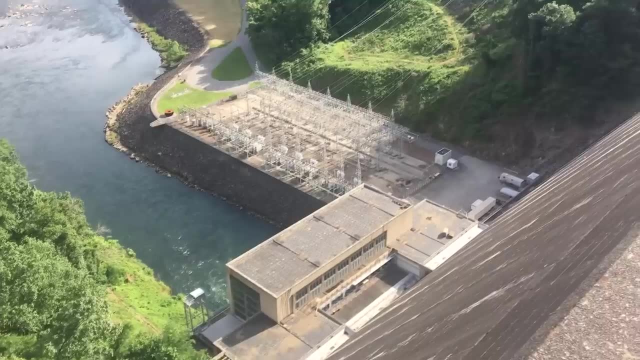 to reduce the current and still get the same amount of power is to increase the voltage. So that's just what we do. Transformers at power plants boost the voltage up to 100,000 volts, and sometimes much higher, before sending electricity on its way over transmission lines. 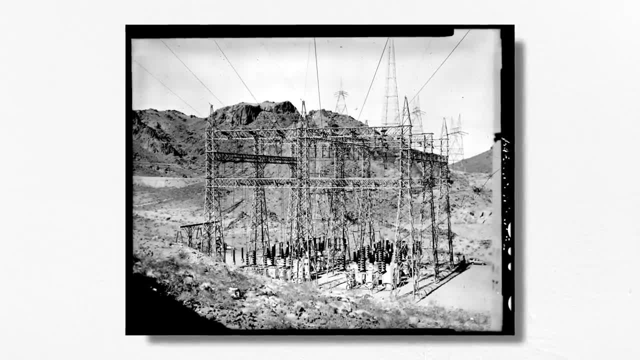 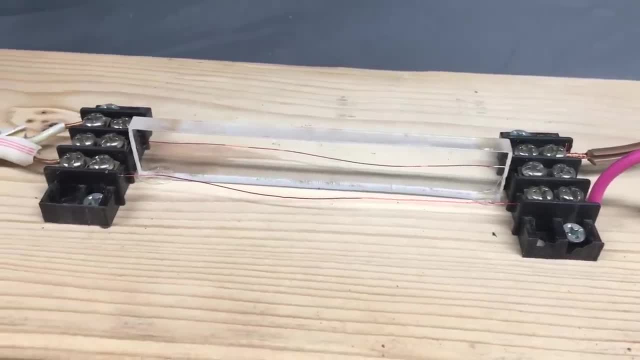 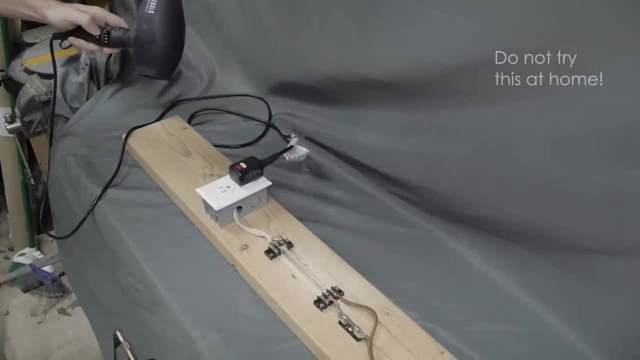 This lowers the current in the lines, reducing the wasted energy and making sure that as much power as possible makes it to the customers at the other end. This simple demonstration illustrates the concept. If I try to power a hairdryer using these thin wires, it's not going to work. The current required to power the dryer is: just too high. It creates so much heat that the wires completely melt. That heat represents wasted energy. But if I first boost the voltage up using this transformer and then step it back down on the other side of the thin conductors, they have no problem carrying the power up. 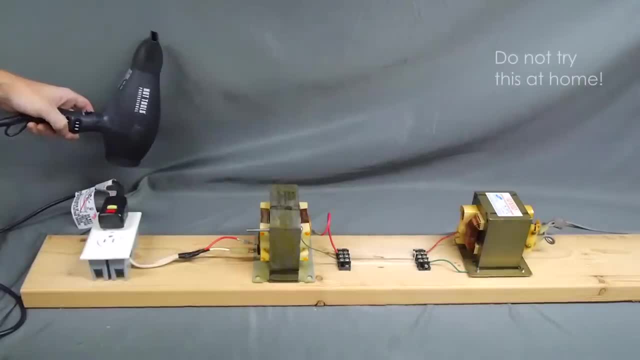 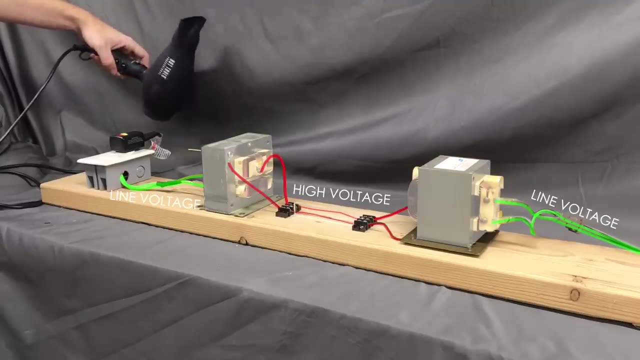 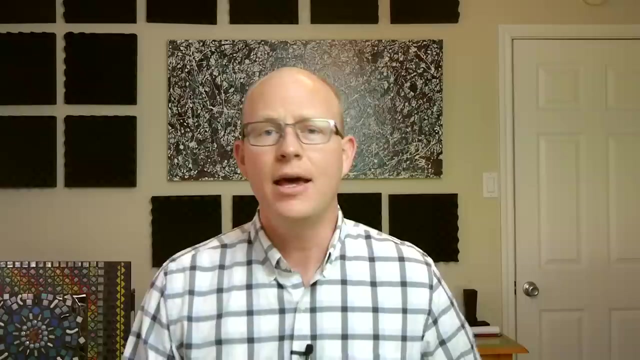 We've essentially swapped high current for high voltage, making the conductors more efficient at carrying power. What we've also done, though, is make things much more dangerous. You can think of voltage as electricity's desire to flow. High voltage means that the 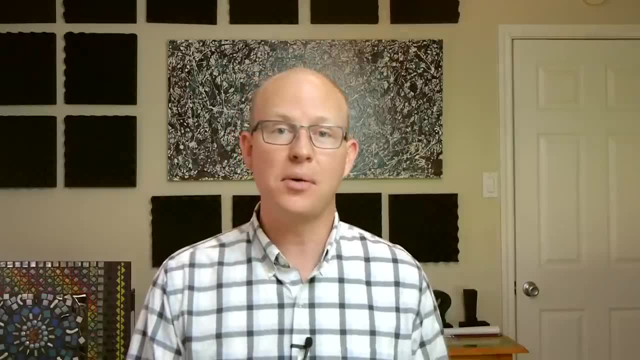 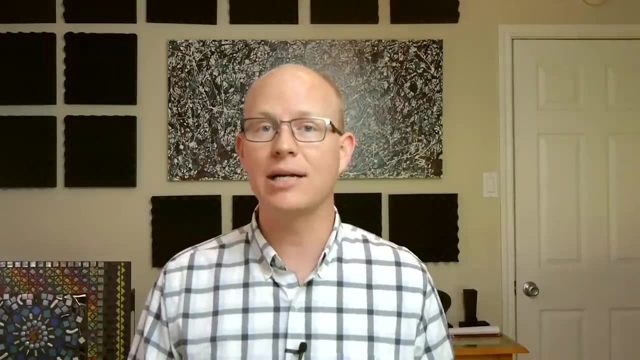 power really wants to move and will even flow through materials we normally consider non-conductive, like the air. Most people designing high-voltage transmission lines have to make sure the lines are safe from arcing and other dangers that come with high voltage. Most long-distance power lines 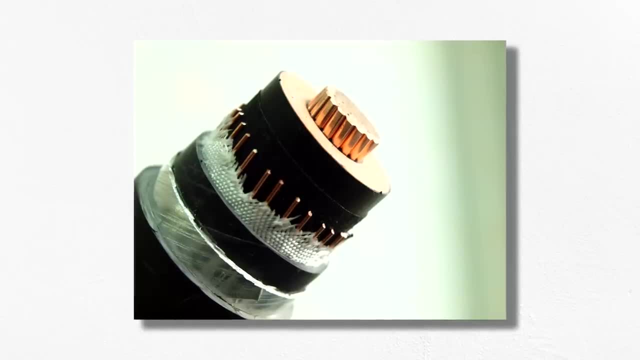 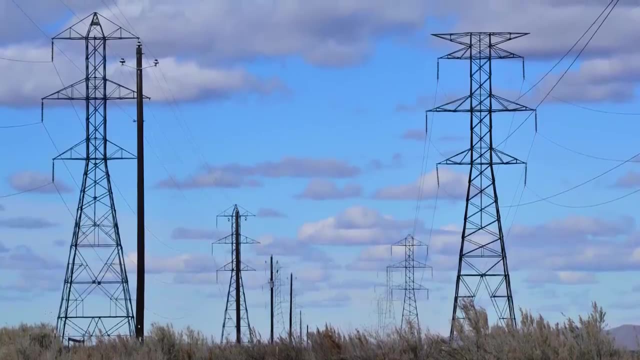 don't use insulation around the conductors themselves. Insulating in this way would have to be so thick it wouldn't be cost-effective. Instead, most of the insulation comes from air gaps or simply spacing. everything far enough apart Transmission towers and pylons. 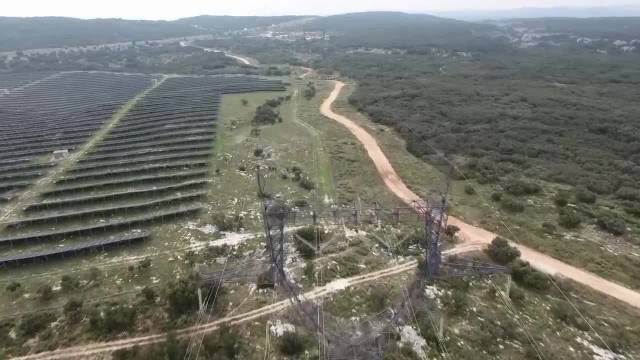 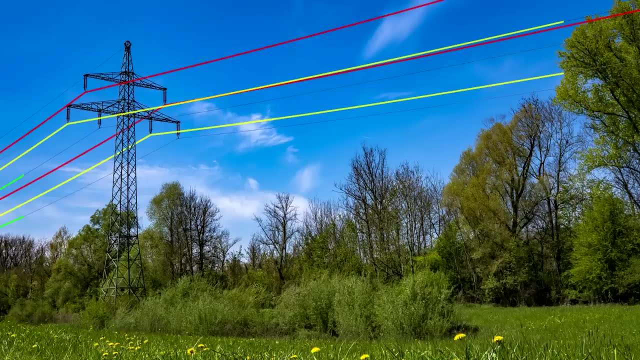 are really tall to prevent anyone or any vehicle on the ground from inadvertently getting close. They're close enough to the conductors to create an arc. Bulk electricity is transmitted in three phases, which is why you'll see most transmission conductors in groups of three. Each phase is spaced far enough, apart from the other. 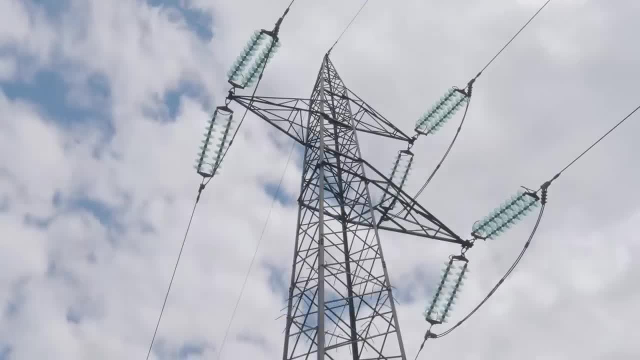 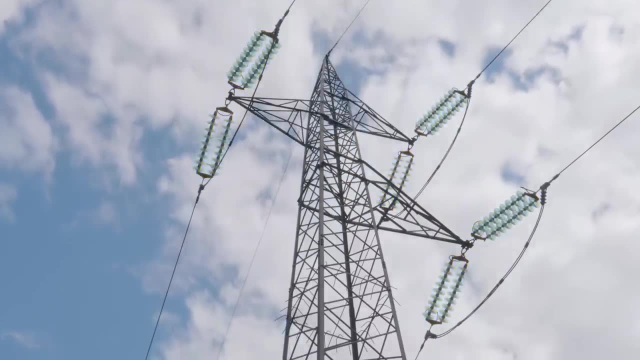 two. to avoid arcing between the phases, The conductors are connected to each tower through long insulators to keep enough distance between energized lines and grounded pylons. These insulators are normally made from ceramic disks so that if they get wet, electricity. 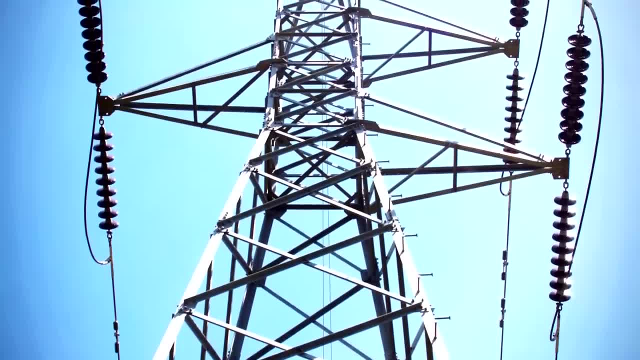 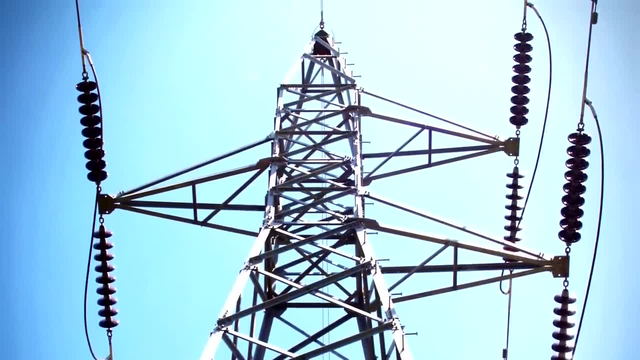 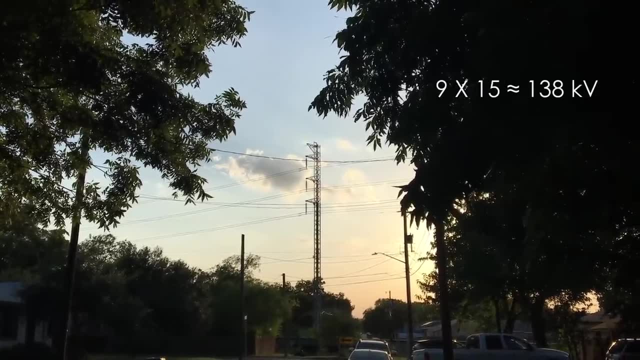 leakage has to take a much longer path. These disks are somewhat standardized, so this is an easy way to get a rough guess of a transmission line's voltage: Just multiply the number of disks by 15.. For example, this line near my house has 9 disks on each insulator and I know it's a 138 kilovolt line. 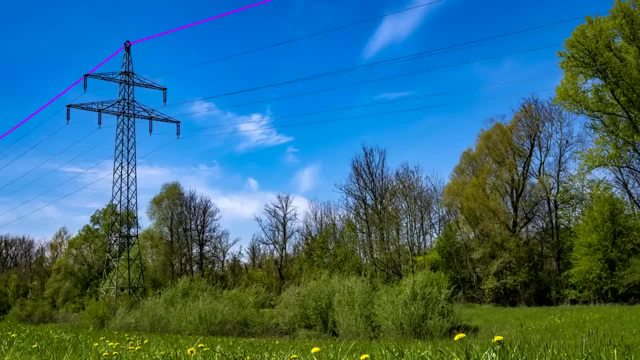 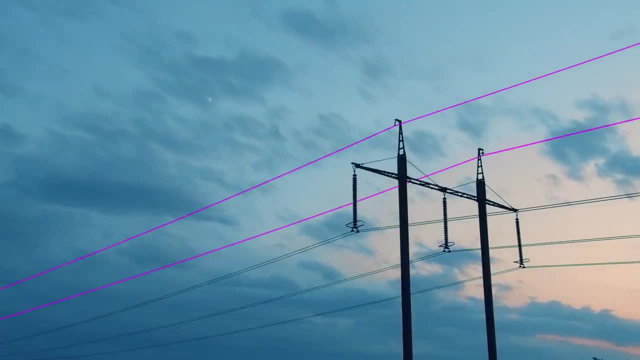 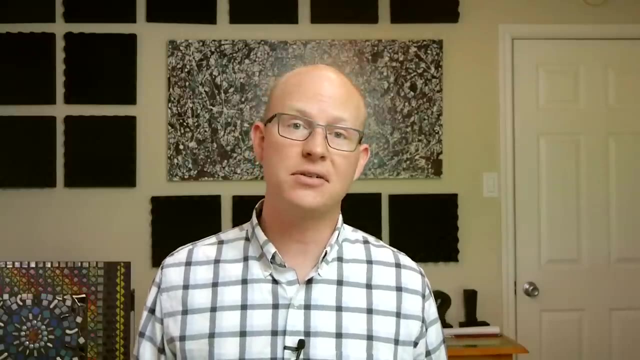 You'll also often see smaller conductors running along the top of transmission lines. These static or shield wires aren't carrying any current. They're there to protect the main conductors against lightning strikes. High voltage isn't the only challenge, though, associated with electrotransmission lines, Just selection of the conductors themselves. 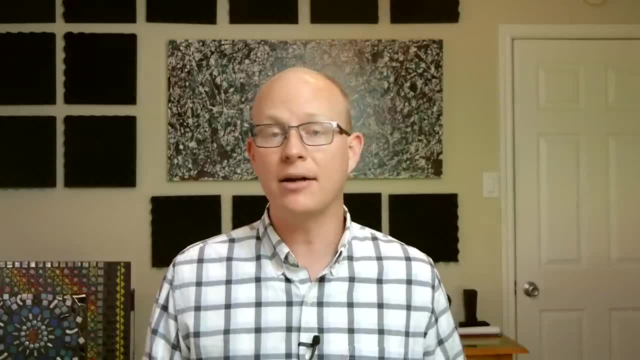 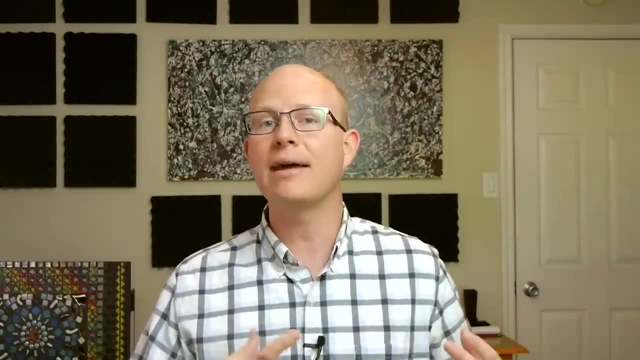 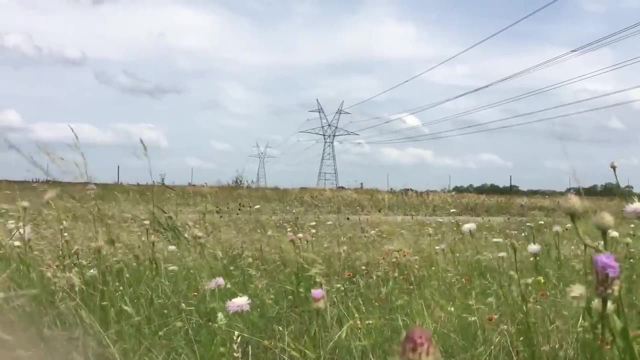 is a careful balancing act between strength, resistance and other factors. Transmission lines are so long that even a tiny change in the material or size of the conductors can have a major impact on the overall cost. Conductors are rated by how much current they can pass for a given rise in temperature. 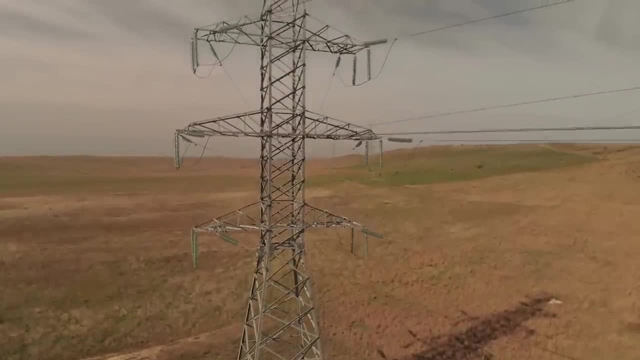 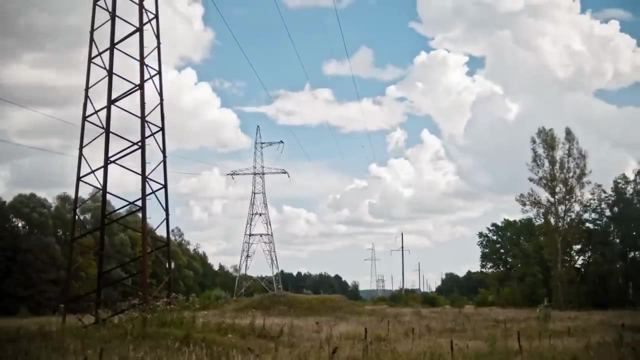 These lines can get really hot and sag during peak electricity demands, which can cause problems if tree-bred conductors are too hot. If they're too hot, they can cause problems if the tree branches are too close. Wind can also affect the conductors, causing oscillations that lead to damage or failure. of the material. You'll often see these small devices called stockbridge dampers to absorb some of that wind energy. High voltage transmission lines also generate magnetic fields that can induce currents in parallel conductors like fences and interfere with magnetic devices. so the height of the tower is sometimes set to minimize EMF at the edge. 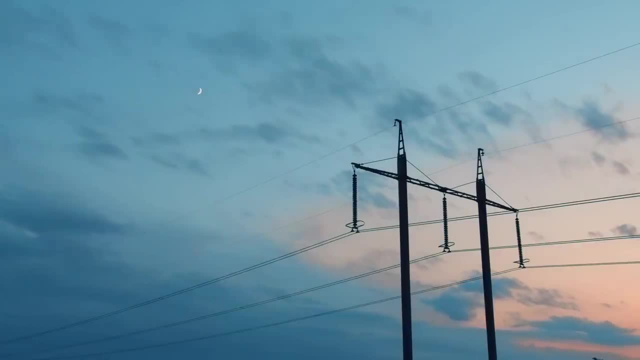 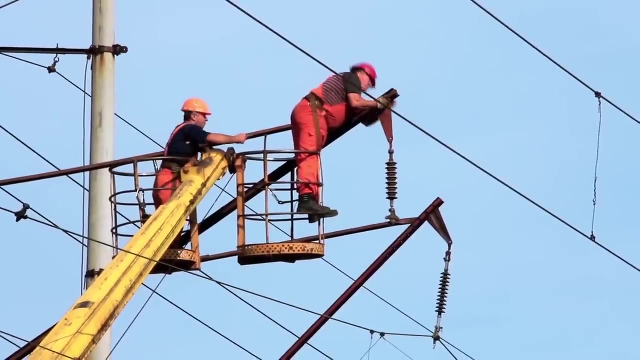 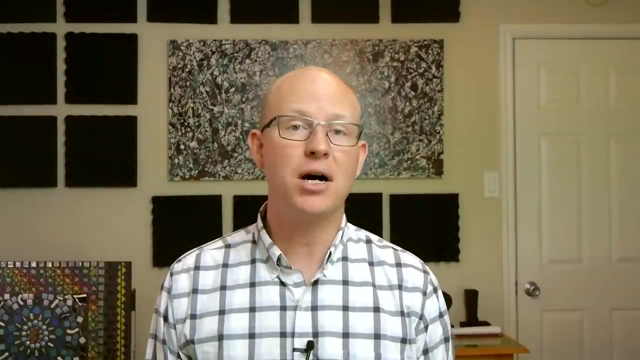 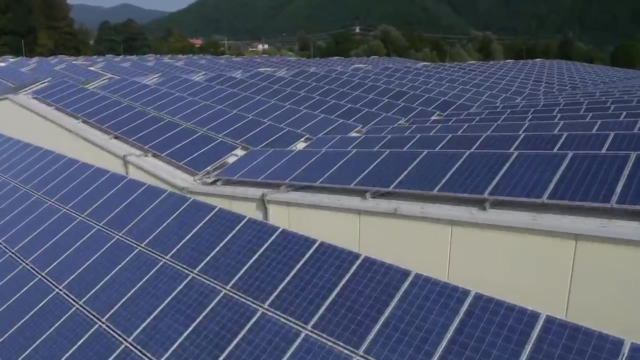 of the right-of-way. In certain cases, engineers even need to consider the audible noise of the transmission lines to avoid disturbing nearby residents. Power Grid: Even with all those considerations, the classic model of the power grid, with generation far away from populated areas, is changing. The cost of solar panels continues to drop, making 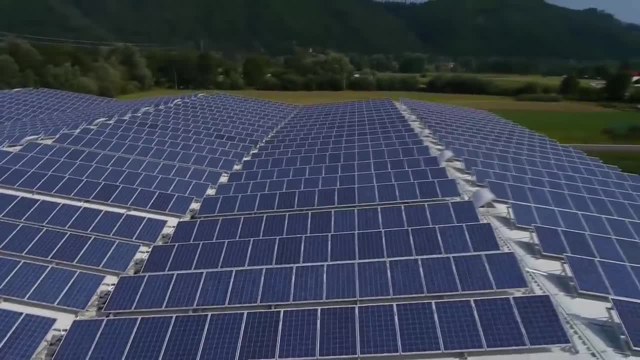 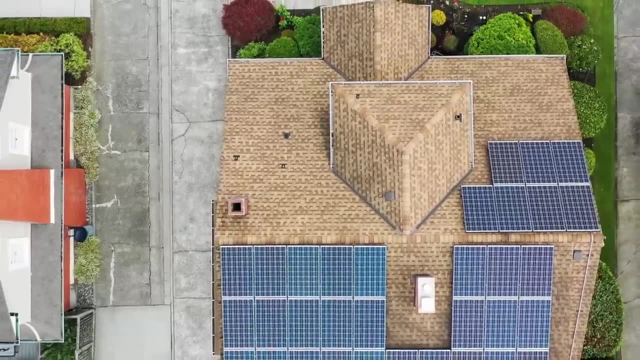 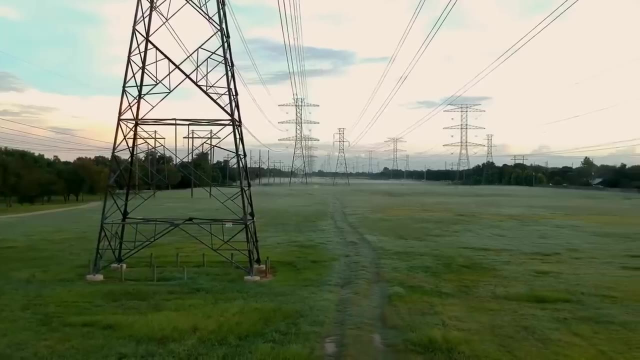 it easier and easier to produce some or all the electricity you use at your own house or business, and even export excess energy. This type of local generation happens on the distribution side of the grid, often completely skipping large transmission lines On the other side of the coin, the energy marketplace. 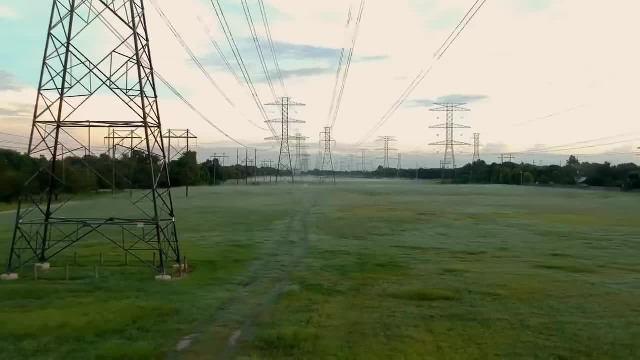 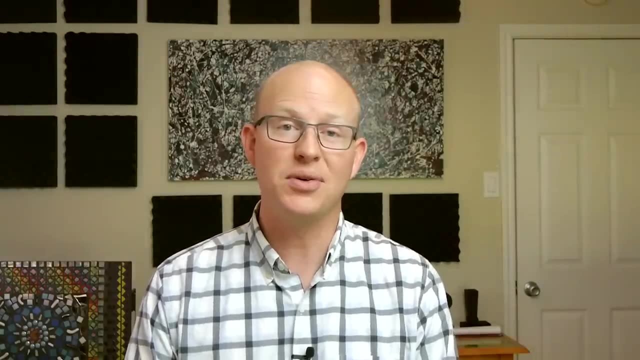 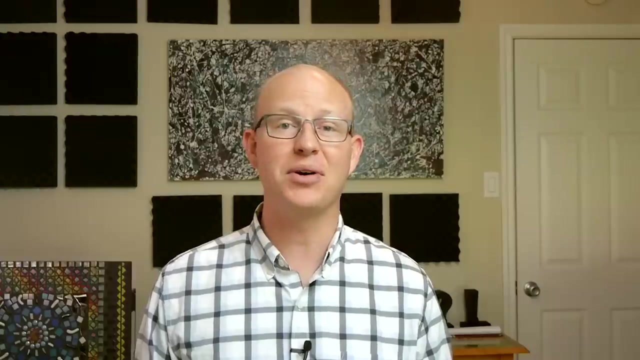 is changing as well, and grid operators are buying and selling electricity across great distances. Electrical transmission lines may seem simple, the equivalent of stretching an extension cord across the sky, but I hope this video helped show the fascinating complexity of even the seemingly innocuous part of our lives. 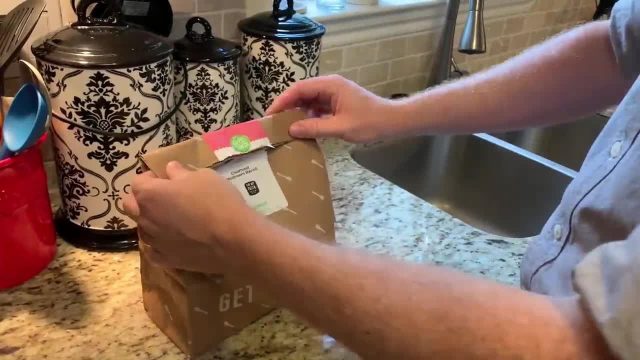 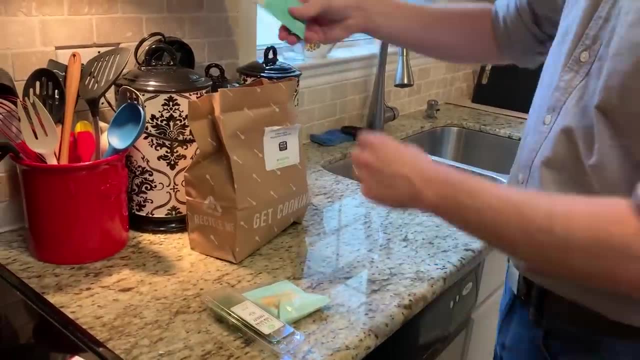 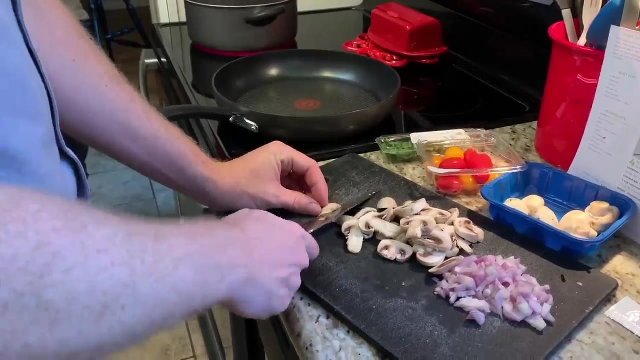 This is a segway between electrical infrastructure and my favorite meal delivery kit, HelloFresh, and this is my wife and I trying to film ourselves making dinner. Spending time in the kitchen is one of our favorite things to do together, and HelloFresh makes it super fun to cook and eat dinner together without the chore of planning meals.